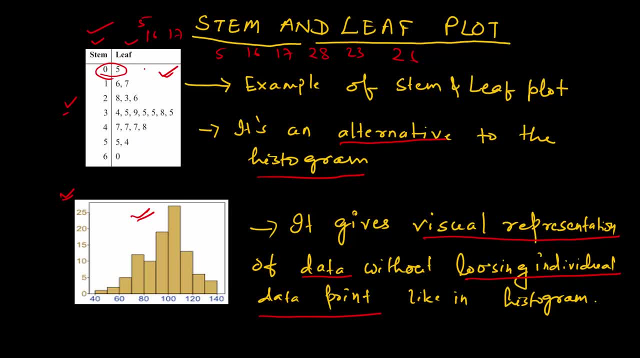 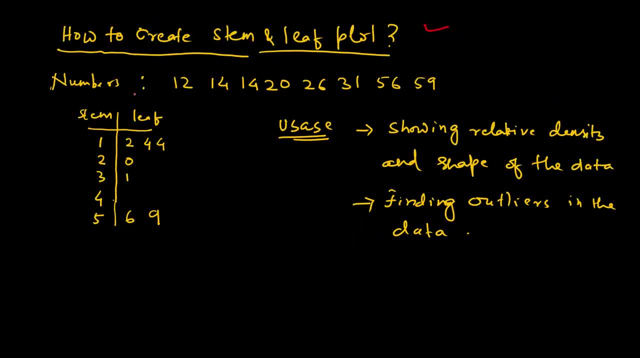 construct this series again into leaf, stem and leaf. We'll just learn in the next slide. So how do we create this stem and leaf plot? Well, let's take an example here. So I've got a number series and the first thing to do is that- to sort it. 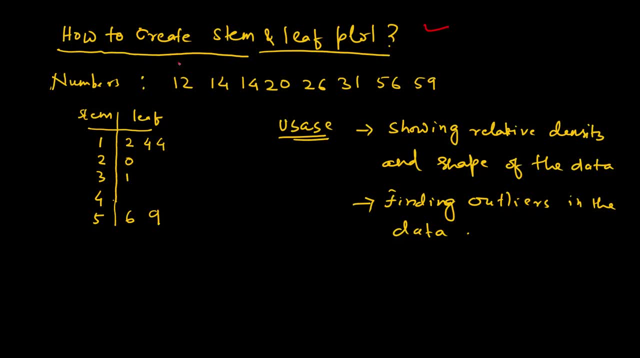 in ascending order right. So the number series is from 12, 14, and that another 14, 20,, 26,, 31,, left a 6 and 59. Now this series we want to represent on the stem and leap plot. So how do we do that? So first notice what is in the leftmost side of. 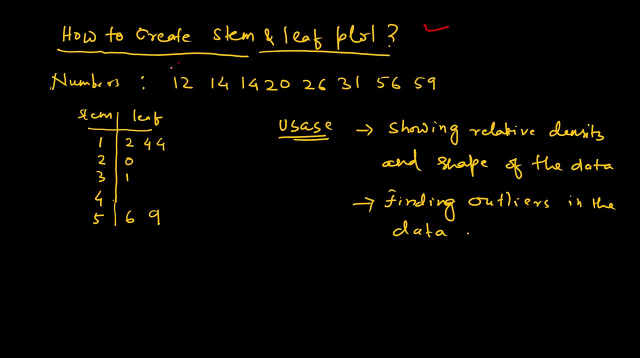 the number, like in this case the decimal number. it's one again here. it's also one, one, two, two and three, five and five, right. so this is the rest in decimal number. so what we'll do is that we'll take the extreme number or the first digit of the 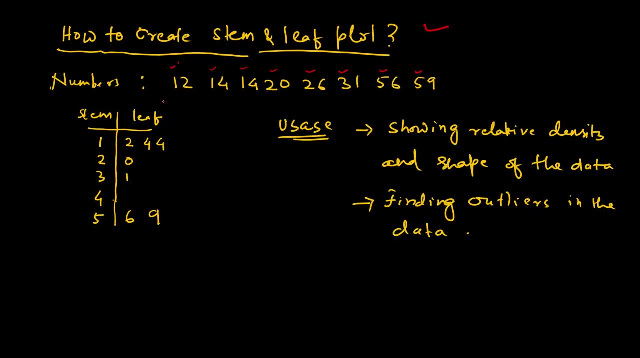 number and we call it a steam, and it starts with one and ends at five. so in between we have got the four is missing, so we have one, and then we have two, three, there is no four, and then we have five. so we, what you do is that we put. 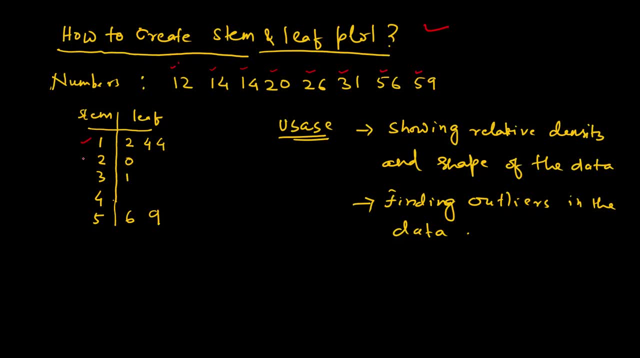 this numbers side and we calling it a stay. so we put one, two, three, four and five. remember that we do not have four, but it's still. we need to put four. we cannot have a gap, so we need to put four over there. then against one, how many? 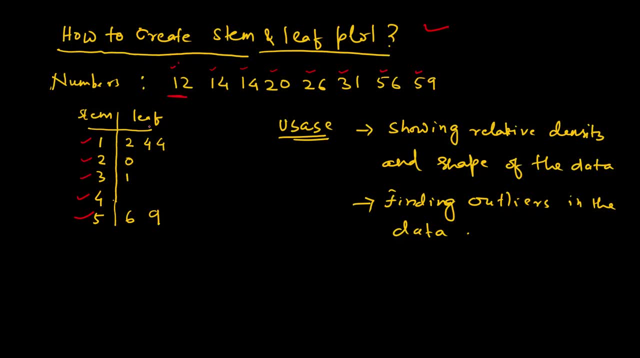 numbers are there. well, in 12 you have got one and two, then one. then in the leaf portion I put two: okay, and then the next number is 14. so what I do is that right next to that I put four. that's how we understand. so one, two, first number, and then one, four. 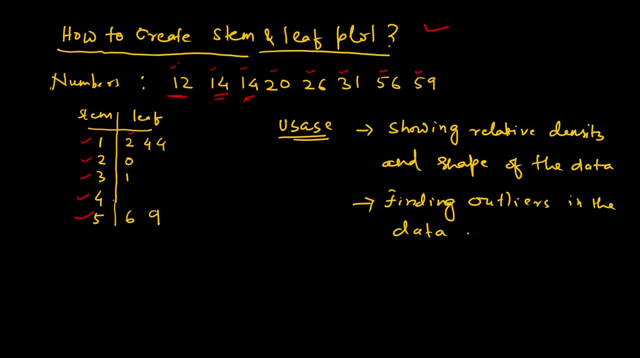 then we have got another 14, so that is again one four, and the next one is 20, so we go to the one step below and then, against two, we we got this zero right, so we'll put six over here. yeah, I just missed that. okay, so we have 20 and then